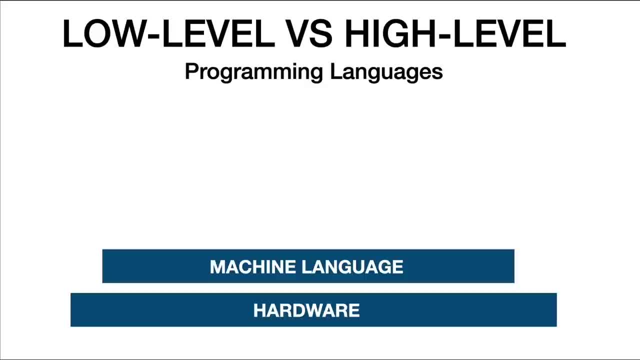 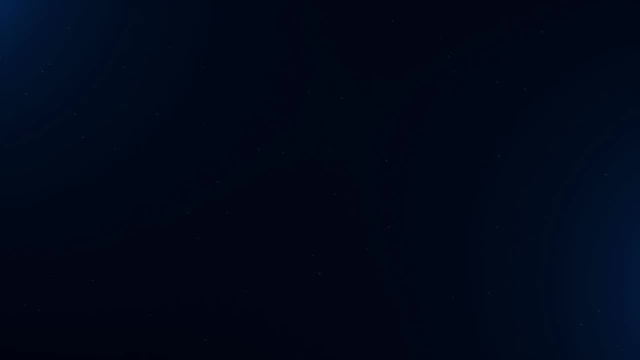 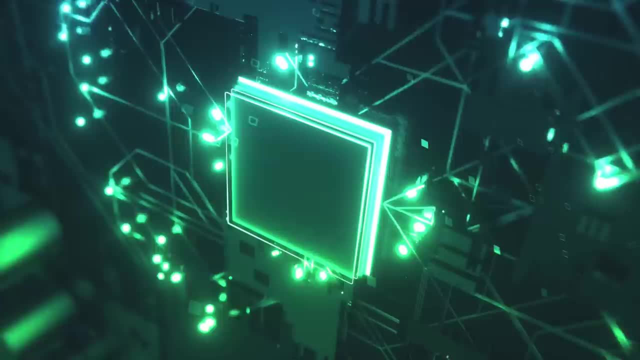 central processing unit, And these instructions are strictly numeric and they're in the form of zeros and ones, which is called binary. Machine code can also be represented as hexadecimal, so it's easier for humans to read. But ultimately machines only process zeros and ones, because those it 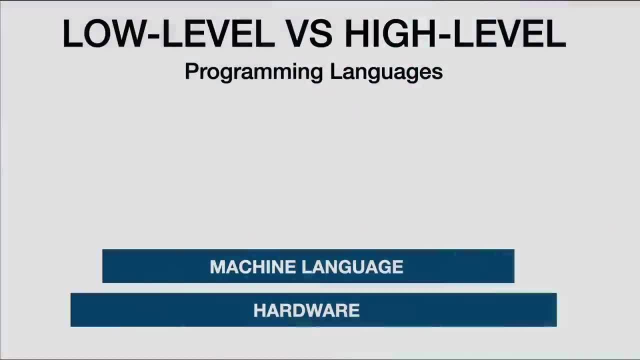 represents an electrical state that's either on or off. All right now programmers don't write machine code, at least anymore. I guess you could, but it would be very tedious and very error prone, And I don't think there's many companies hiring senior machine code developers. 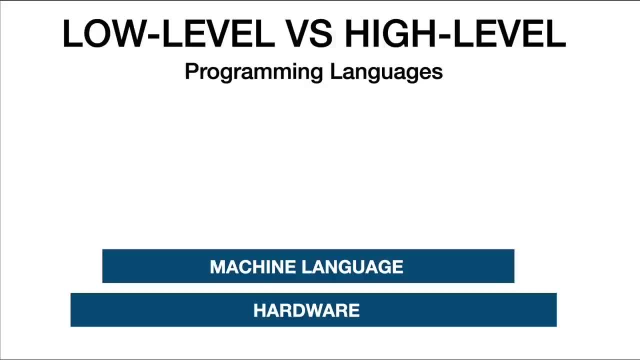 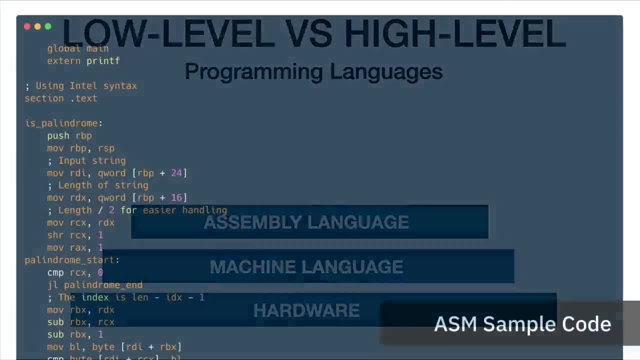 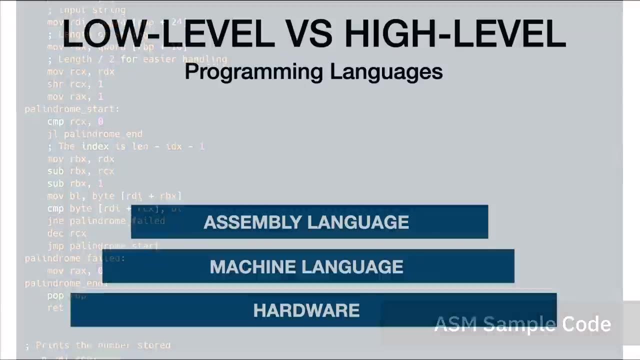 All right. So the next level we have, up from that, I should see the next language we have is called assembly language or ASM or just assembly. And assembly uses numbers, symbols and abbreviations as opposed to just ones and zeros like binary machine code. And assembly code isn't actually compiled like some of. 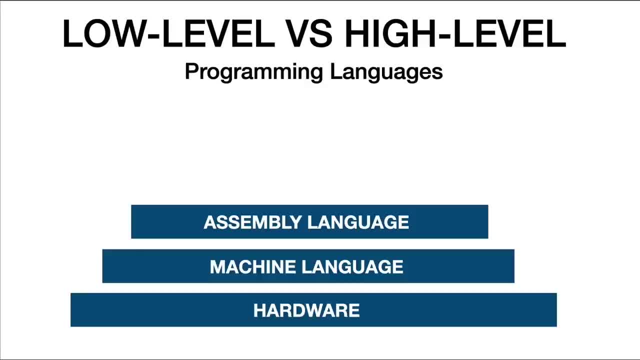 the higher level languages. It's converted or assembled into executable machine code by something called an assembler. Compiling, which I'll talk about soon, is a much more complicated task than assembling. A lot more goes into it And you can learn assembly language. 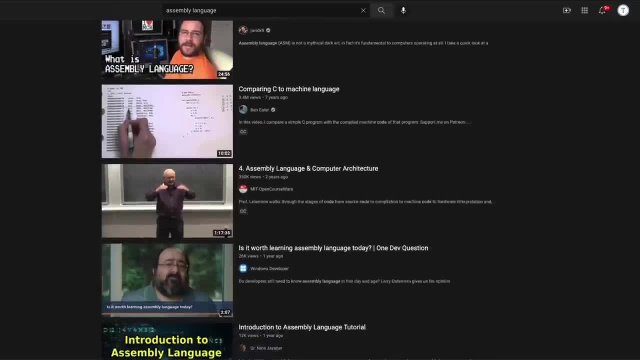 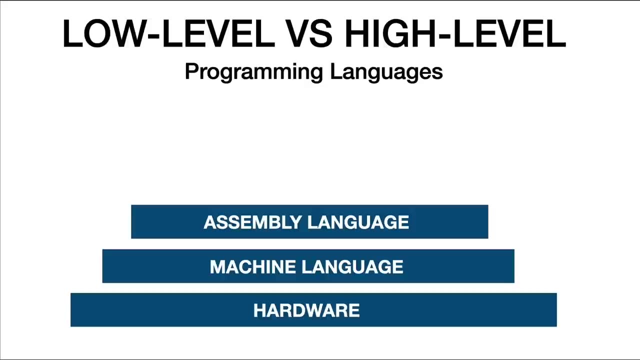 There's YouTube videos, There's even Udemy courses that you can take to learn assembly language, And I do think it's interesting because you really start to understand how software works with the CPU and works with your computer's hardware. Assembly is typically used today to develop software. 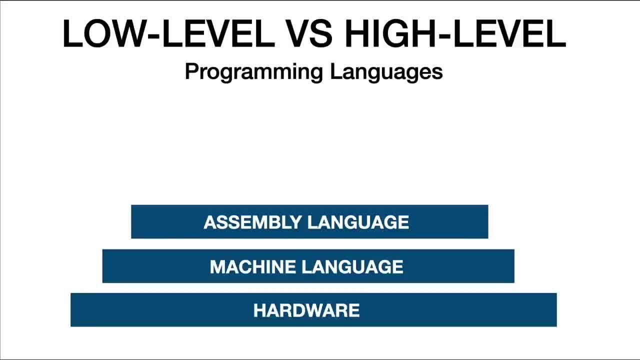 or firmware for embedded systems. Now, from here we have the next level, which consists of a bunch of general purpose languages that are pretty common. Now, in some cases, you'll see charts like this that refer to these as high level languages, languages like C, C++. However, that's when you're comparing it. 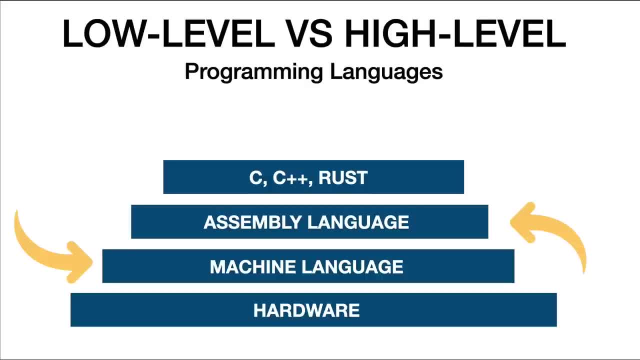 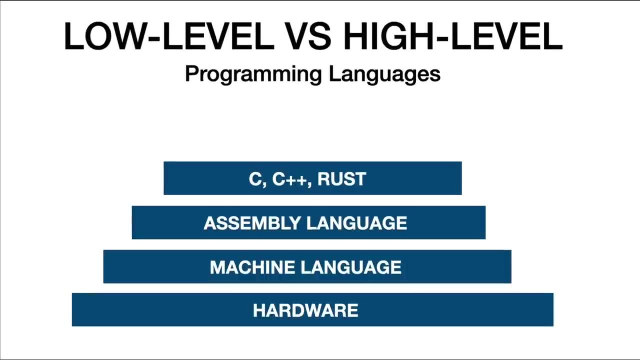 to the whole chart, to machine language, assembly language and so on. These languages are lower than something like Python or Java or Ruby, which we'll talk about later. So let's take a look at C. C is the lowest level general purpose language. The only thing lower than C is: 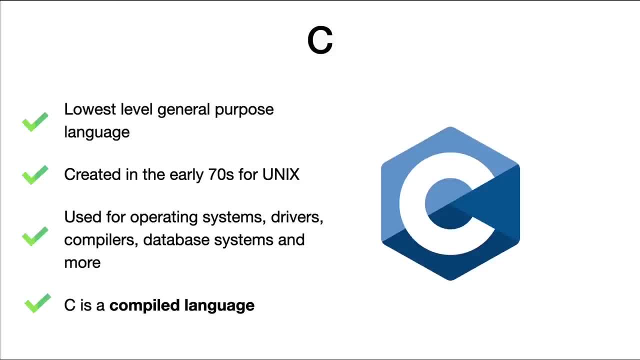 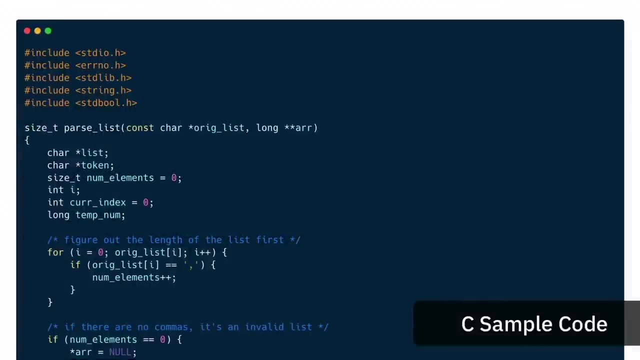 assembly and machine code, And C was created in the early 70s by Denis Ritchie and was actually derived from another language called BEA, And C was used in the development of the Unix operating system. It's a procedural language as opposed to an object oriented one, and it's lower level. 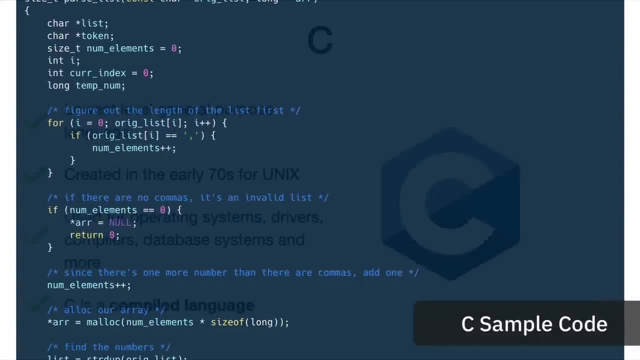 than many other languages. So you do have to manage some hardware resources such as memory allocation, and I'll talk a little bit more about that in the next slide. So C is very route oriented. You can't go off site if you don't know the different farmers- automatic. 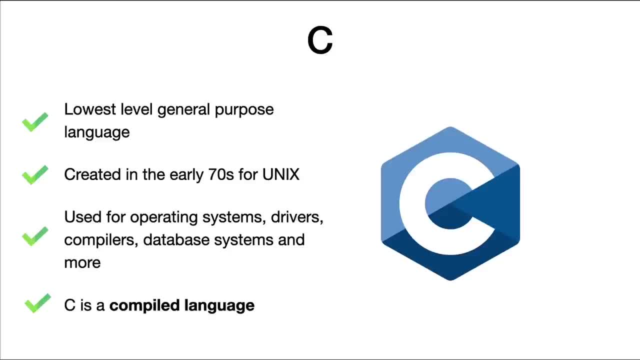 So C is very route oriented. You can't go off site if you don't know the different farmers. automatic powerful. it's used for things like operating systems. the Windows kernel, for instance, is built with C. it's also used to build compilers for other languages. it's used for drivers, database systems and many other powerful programs and C. 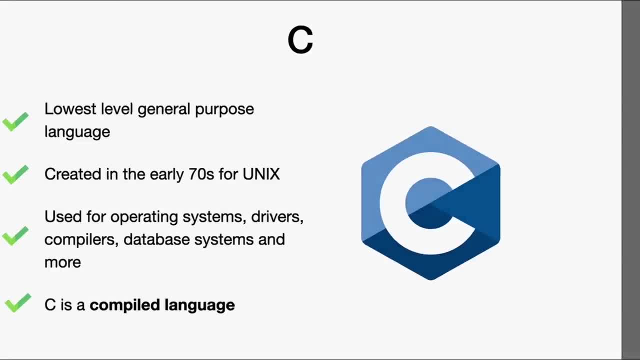 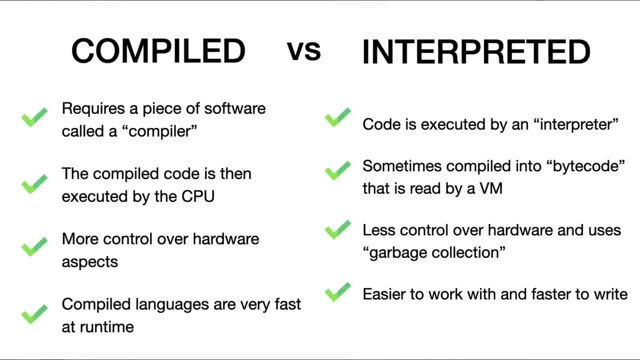 is also a compiled language. so before we move to the next language, let's talk about compiled versus interpreted languages. so a compile language requires a piece of software called a compiler which will compile the code that you write with a language like C down to instructions that the machine 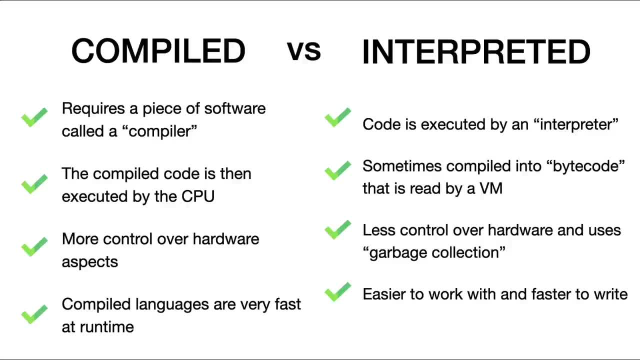 understands. so the compiled program is not human readable. it's meant for them, the machine, and it's executed by the CPU. now, usually with lower level compiled languages such as C, you have to manage your memory. so memory allocation, CPU usage. you have more access to the hardware, but of course it's more. 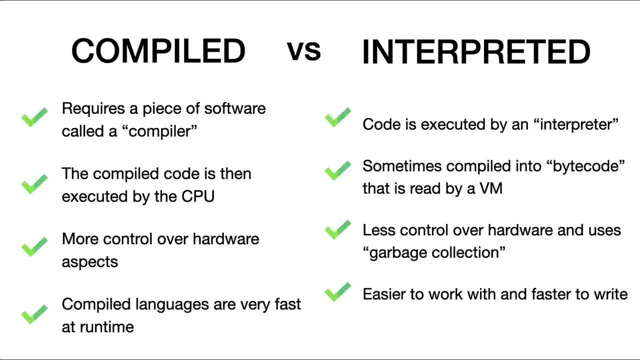 difficult to work with. with an interpreted language, the source code is not directed to the computer. it's directed to the computer. it's directed to the machine code. there's more abstraction to it, and a program called an interpreter reads and executes the code. in some languages like Python and Ruby are first. 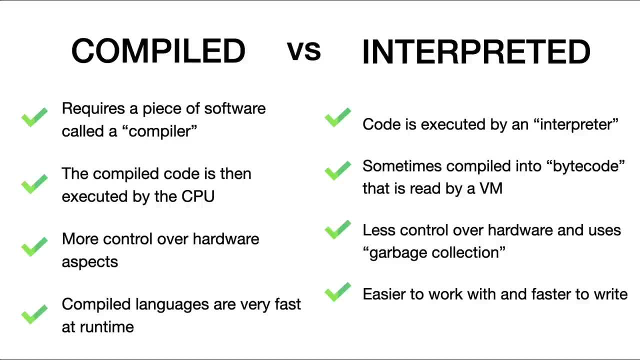 compiled into some sort of bytecode, which are binary instructions that are executed by a virtual machine such as the Python virtual machine. technically they do have a compile step, but they're not being compiled directly to machine code like with, with a lower level language like C, so usually refer to those as interpreted or scripting languages. now, 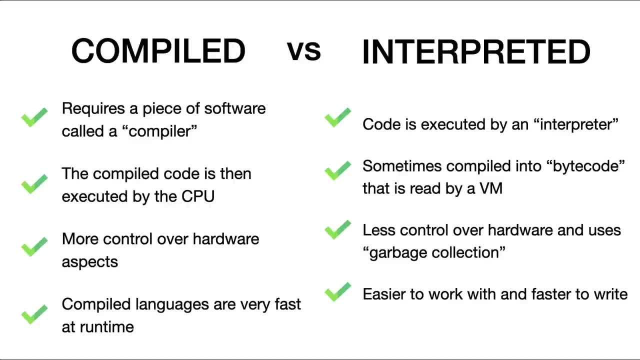 interpreted languages are typically easier to work with and allow you to write code faster, so there's a fast write time. however, there's more abstraction than with a compiled language, where your code is simply compiled directly into machine code and executed. so this makes programs faster at runtime for a compiled languages. and, of course, this isn't all you're gonna. 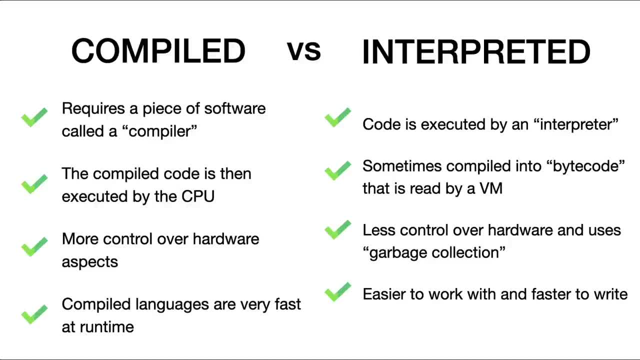 look at when choosing a language, and it's incredibly important to have a. It's just good to know the difference. So the next language we're going to look at is C++, which is another lower-level language that was created in the 80s. 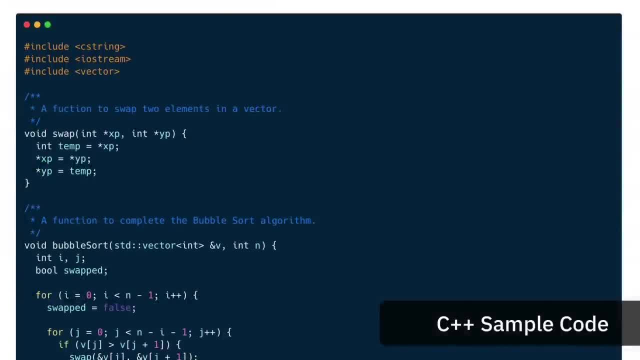 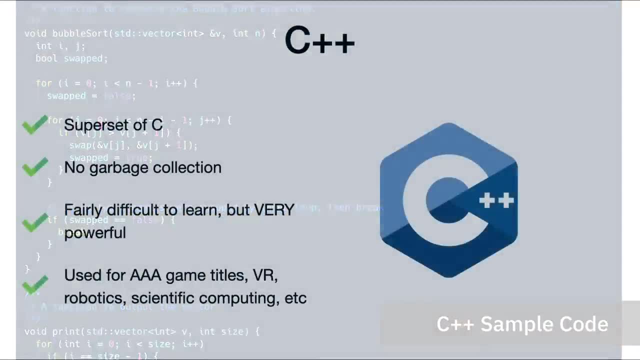 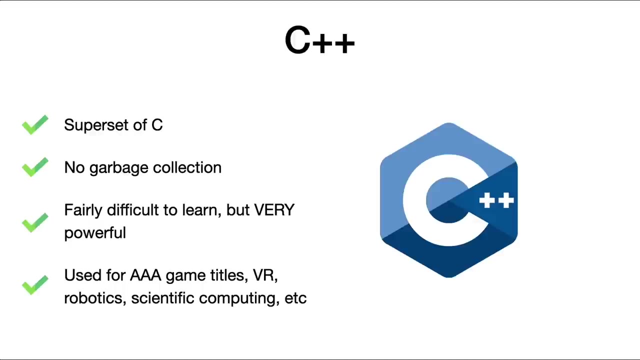 And it's actually a superset of C, meaning that it is essentially C but it has a bunch of extra tools. So C++ is actually object-oriented, which is a coding paradigm based on the concepts of objects And, like I was talking about in the last slide, both C and C++. there's no what's called garbage collection, which means that you have to manually allocate and free memory within your code. 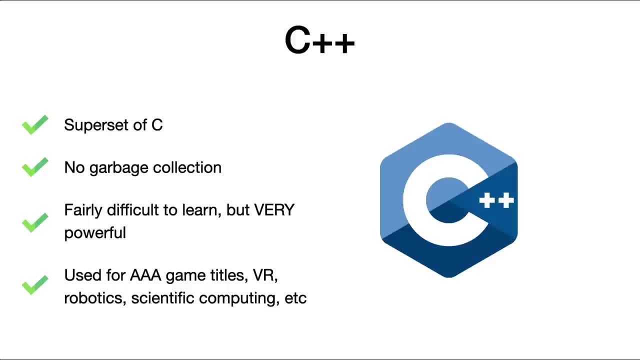 So C++ is an incredibly powerful language. It's used to build things like AAA gaming titles, operating systems. It's used in VR, robotics, scientific computing and stuff like that. So if you're interested in those types of that part, 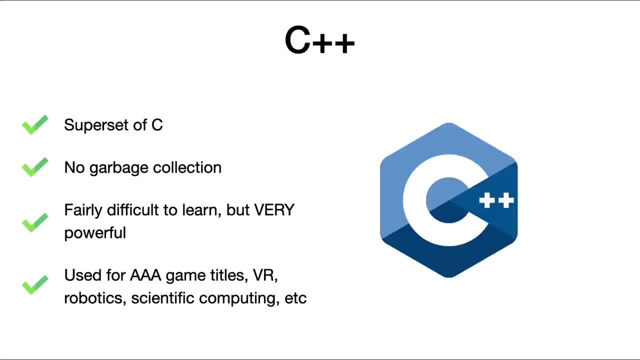 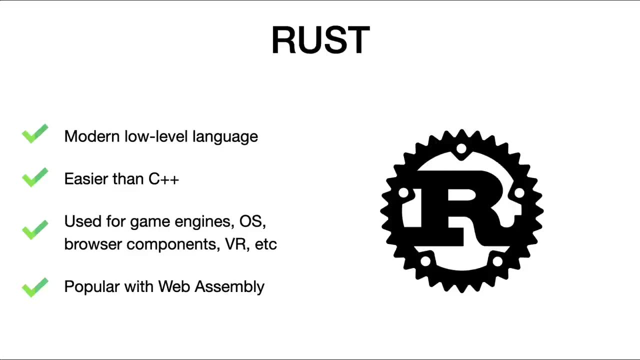 If you're interested in that type of technology, then C++ might be something to look into. All right, so Rust or Rustlang, is a relatively new low-level and high-performance language that provides higher-level capabilities And it provides protection to keep you from making mistakes with memory allocation. 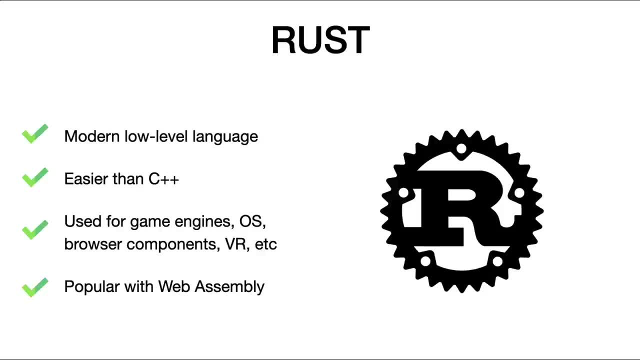 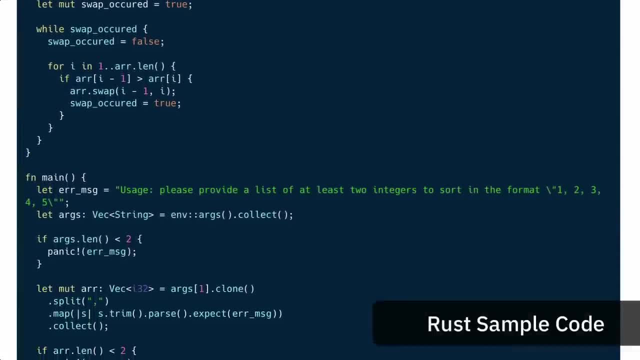 So there is no garbage collection, but there is protection built in, more so than something like C or C++, And Rust can be used for game engines. It can be used for game engines, operating systems, browser components, VR and much more. 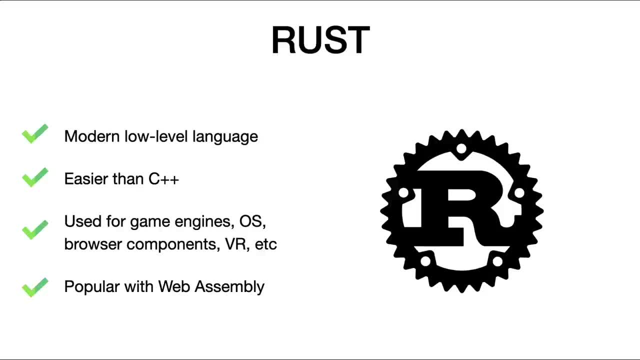 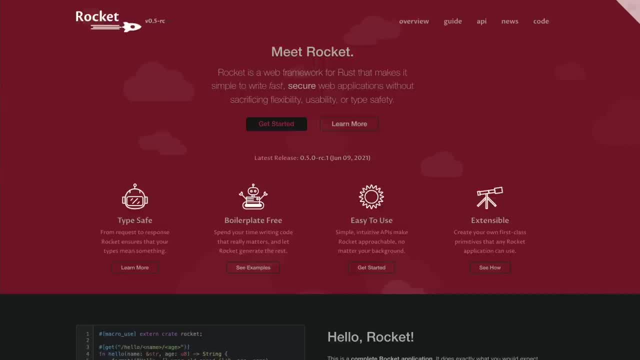 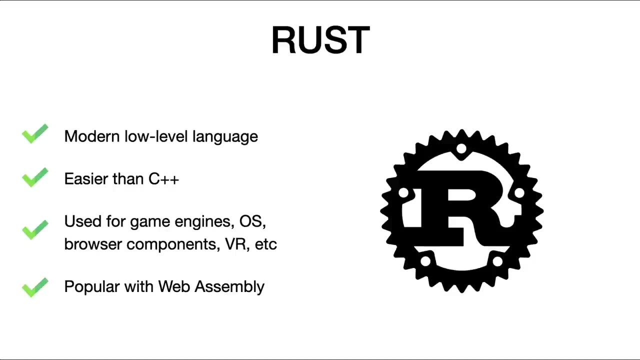 And it can be used to create web servers and used in the back end for web development. You can create APIs and microservices with Rust. It has some frameworks, like Rocket, which will help you build web applications, And one area that I think Rust is thriving in and will continue to thrive in is WebAssembly. 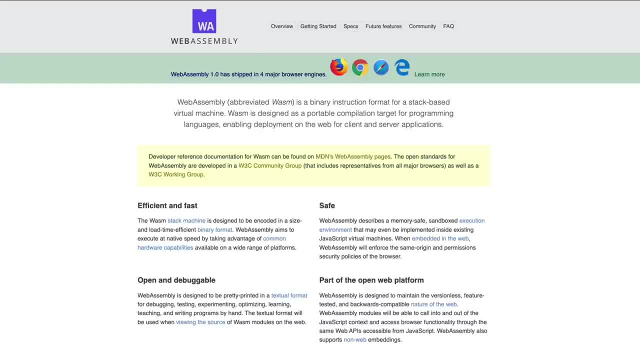 So WebAssembly is a new type of bytecode that can be run in modern browsers And it provides very high performance within the browser, much higher than what JavaScript can give us. So there's a few languages that can be compiled into WebAssembly, including C++ and Rust. 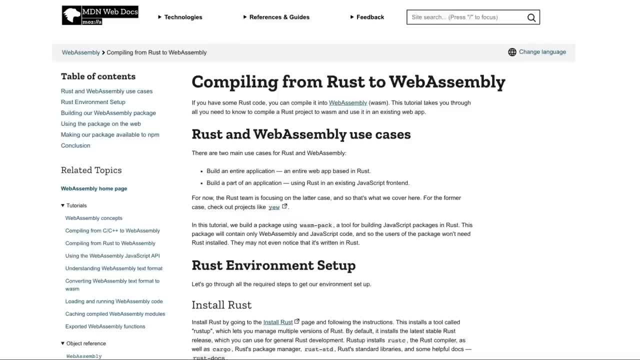 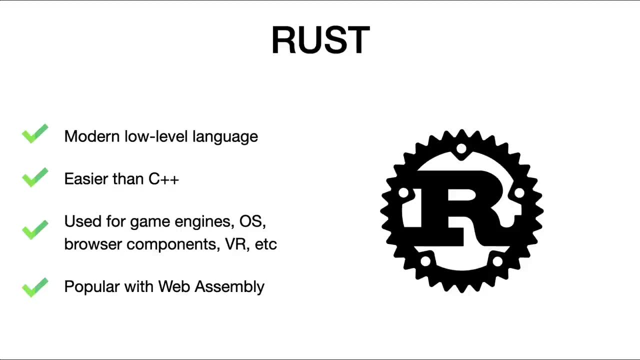 And I think WebAssembly is going to be huge in the future for things like gaming and video tools within the browser. So learning Rust may be a really good idea if you're into that kind of thing. All right, so we're going to move to some even higher-level languages. 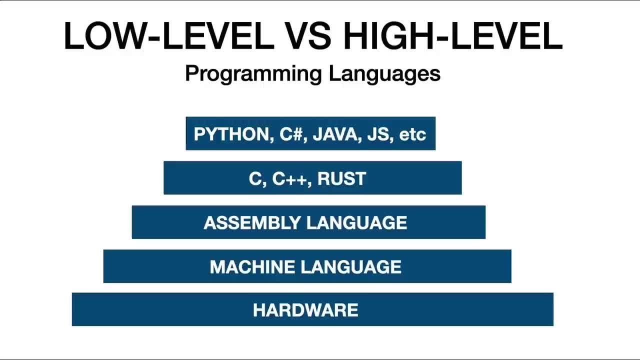 which are most of which are interpreted, So they're not quite as fast in terms of the software you build, but they're generally easier to learn and extremely popular in the industry. Since this channel is focused mostly on web development, these are probably the language that you're going to be choosing from. 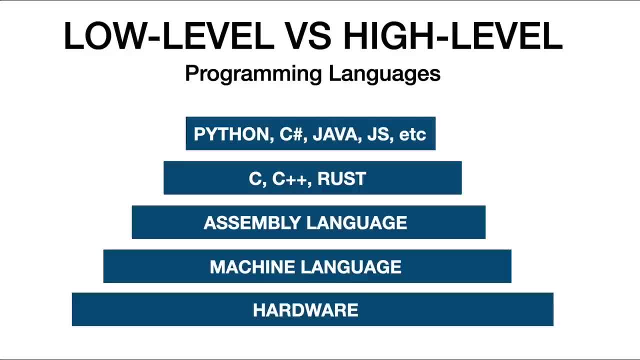 Also, I do want to mention that there are other lower-level languages that are on this level here, such as Pascal, But I don't want to make this video too long, so I'm not going to talk about every single language. I'm going to talk about every single language in existence. 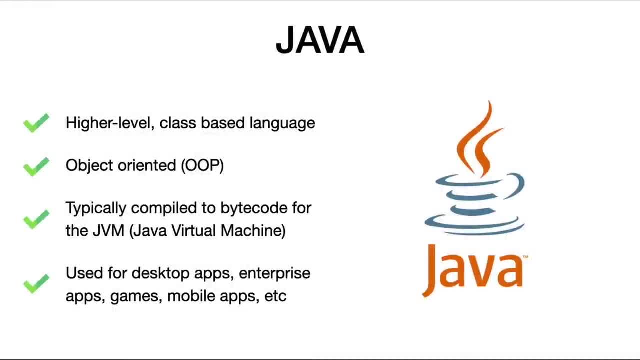 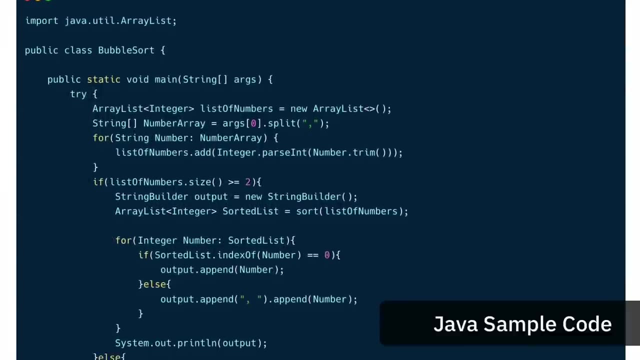 So next we're going to look at Java. So Java is a high-level class-based object-oriented programming language. Everything you create in Java is essentially an object or part of an object, And objects are defined by classes that have variables, which are also called properties and functions, also called methods. 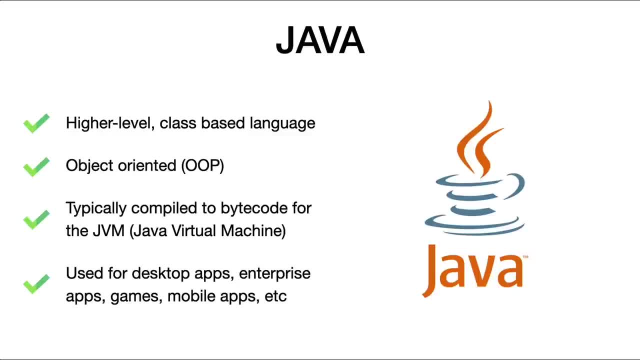 So Java is what's called a write-once-run-anywhere language, meaning that compiled Java code can run anywhere. It can run on all platforms that support Java without the need to recompile. So Java code is typically compiled into bytecode that can run on what's called the JVM or the Java Virtual Machine. 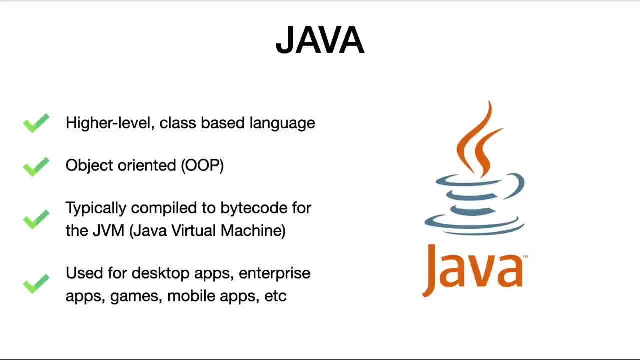 And I'm sure that you guys all have installed the JVM on your computer at one point or another. So Java is used for a lot of different things, including graphical desktop applications, enterprise applications. Java is still pretty popular in big business. It's also used for web servers and APIs. 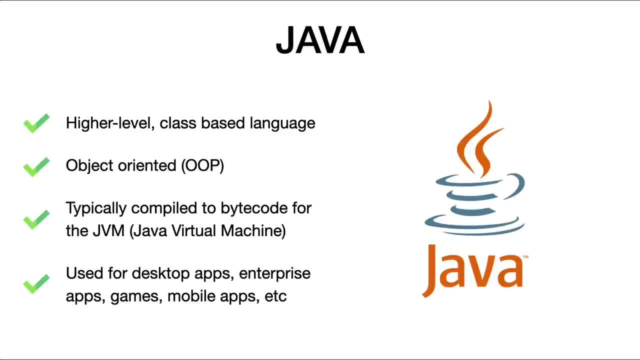 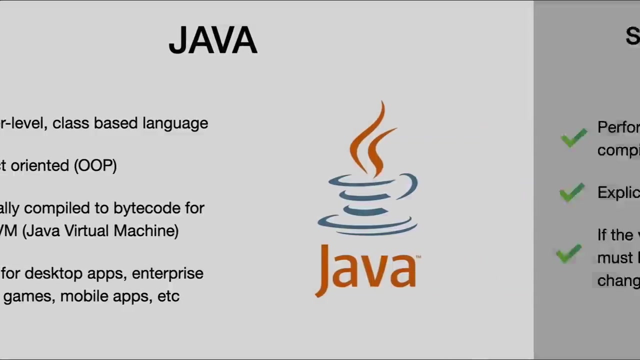 It's used for mobile app development, specifically Android apps. Google uses Java for many of its products. Minecraft was created with Java, And companies like Spotify, LinkedIn, Amazon all use it in one form or another. Java is also statically typed, So this is something else that I wanted to talk a little bit about before moving forward. 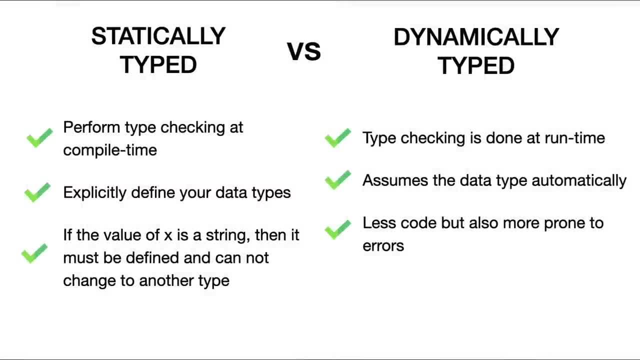 So every general problem is solved. Every general purpose language that we've talked about up to this point is statically typed, And what that means is that the type checking is performed at compile time And we have to explicitly define types for our data within our code. 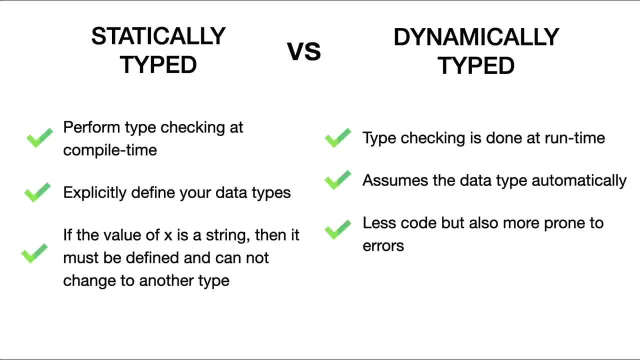 So for our variables and our function returns, if something is a string, we need to define it as a string, and it can't change into a Boolean or some other type. Now, dynamic languages such as JavaScript and Python, which we'll get to soon, do not require us to define types explicitly. 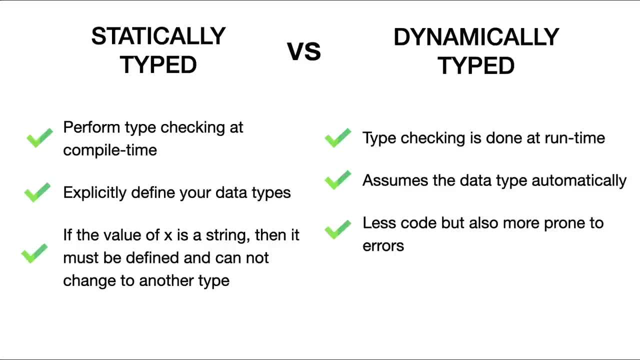 as type checking is done at runtime, So it basically assumes the type automatically or dynamically, As far as. which is better. there's trade-offs with dynamic languages. You don't have to worry about typing everything, so it's less code. However, statically typed languages can be less prone to errors and can be more robust. 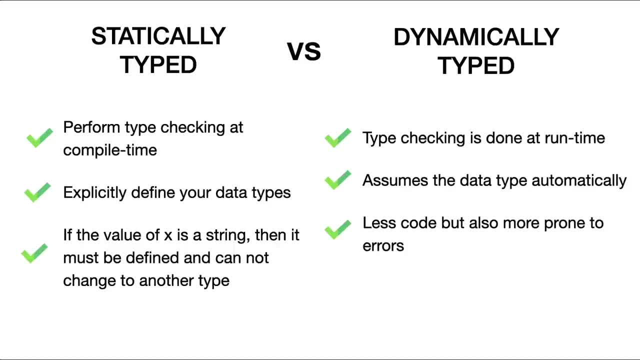 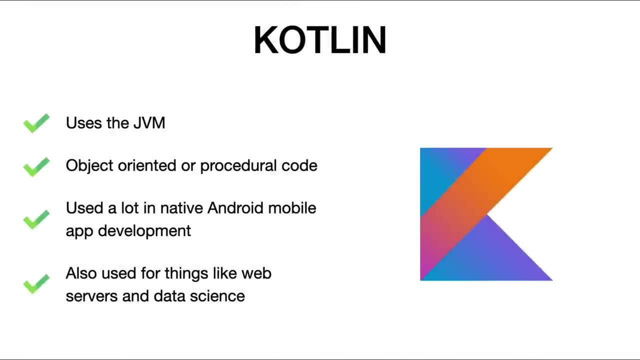 So just keep that in mind, Keep that in mind moving along- And I know that I have a lot of JavaScript developers as viewers, and you can just think of JavaScript versus TypeScript, because TypeScript is JavaScript with static typing, All right. so I wanted to mention Kotlin, right after Java. 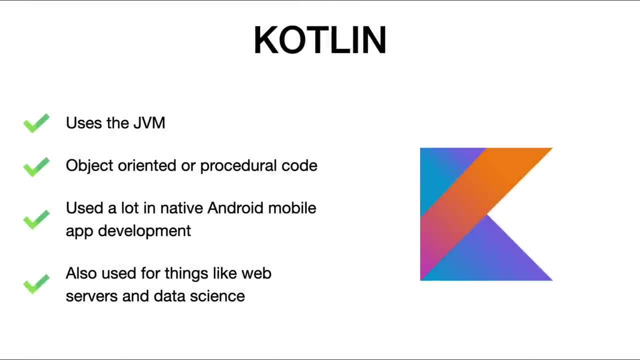 because it also uses the Java Virtual Machine, the JVM, and it's also used for Android apps. In fact, most modern native Android apps are built with Kotlin. If you're looking to learn Kotlin or Java, I'd probably suggest Kotlin because of its popularity. 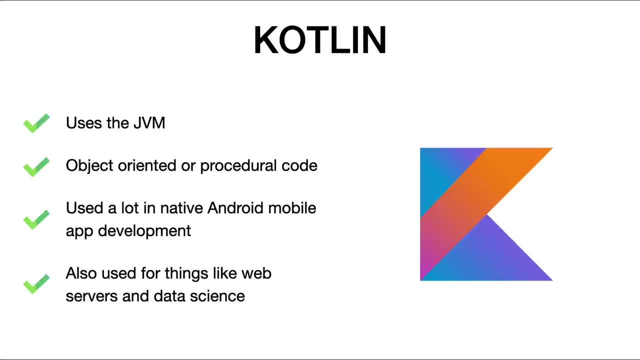 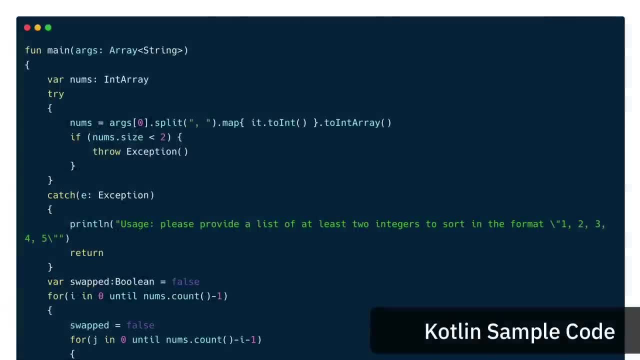 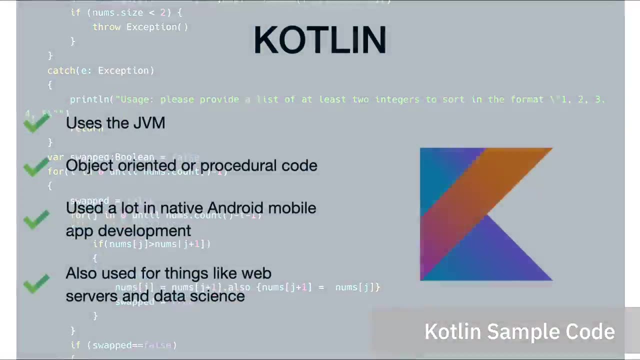 and most people say that it's easier than Java. I don't really have any experience with Kotlin, but it can be used as an object-oriented language or procedural code. In addition to mobile development, it can be used for web servers, data science and much more. 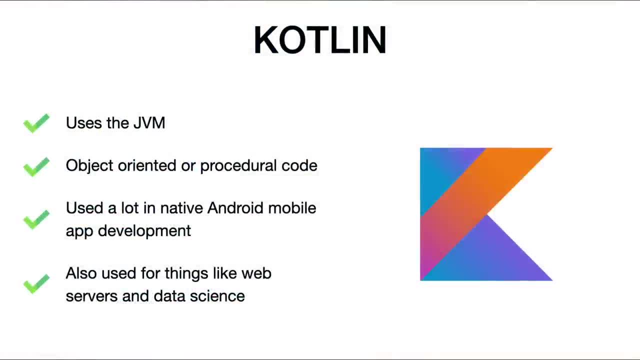 So, as far as who uses Kotlin, you have cache apps, VMware, PlanGrid. these are some examples of services or companies' products that use Kotlin. So next we're going to look at C Sharp, which is another compiled and statically typed language. 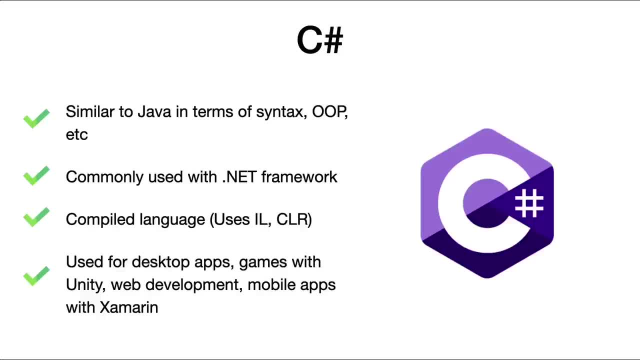 And unlike C and C++, it is fully managed in terms of garbage collection. I know all the different C languages can be confusing, but C Sharp is higher level than the others. It is object-oriented, much like Java. In fact a lot of the systems in Java. 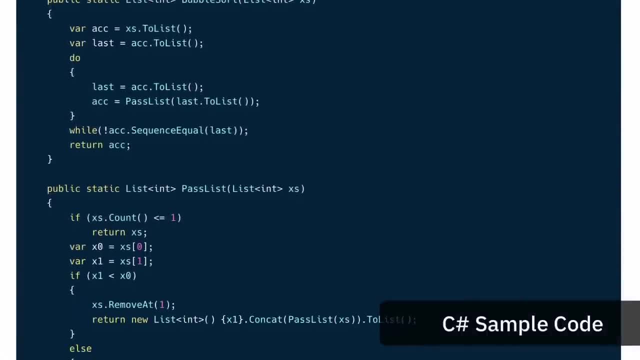 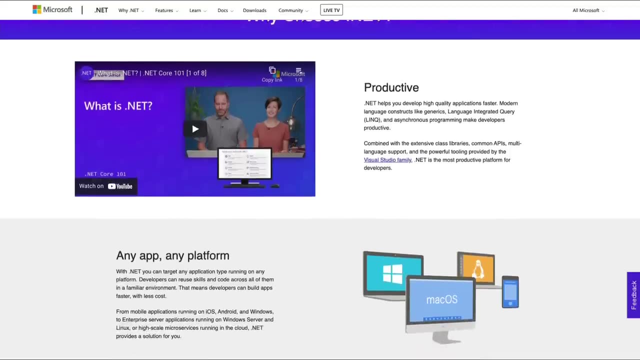 look similar to Java, in my opinion. I've used both. I would most likely suggest C Sharp over Java, though You have the NET framework, which C Sharp can use. You can also use the Visual Basic language as well as F Sharp with the NET framework. 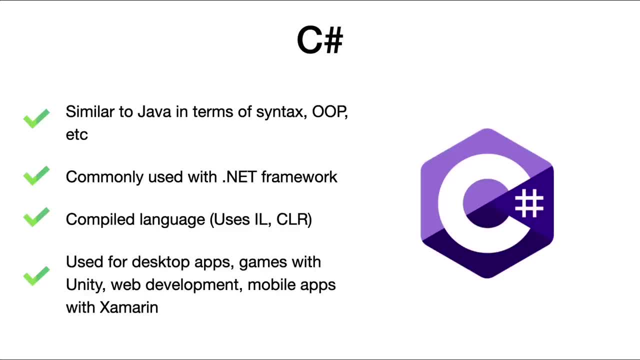 C Sharp is typically called a compiled language, but it isn't compiled directly to machine code. It's compiled into something called IL or C Sharp Intermediate Language, And C Sharp also uses the CLR or Common Language Runtime Environment. So when it is compiled, 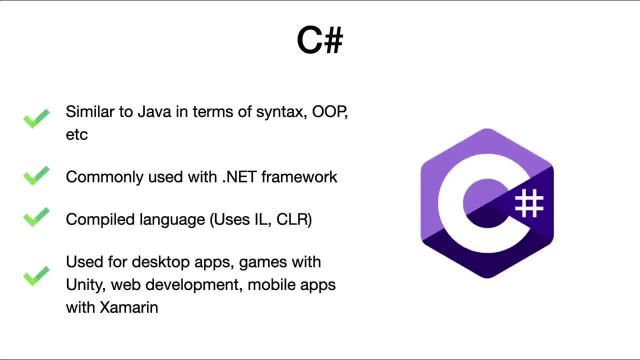 there's just a little more abstraction to the process. C Sharp is used for desktop applications, especially Windows apps. Microsoft did create C Sharp and NET, So they're great tools for building on Windows. C Sharp is also used for web development. 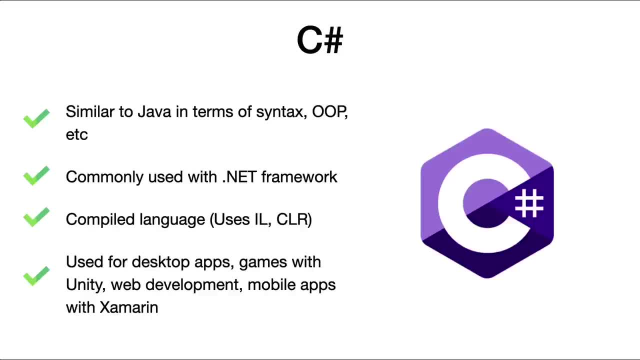 You have the ASPNET MVC framework. It can also be used for gaming along with Unity, and mobile apps along with Xamarin. I think C, Sharp and NET is an excellent choice for a tech stack for many different purposes. Microsoft's Visual Studio IDE. 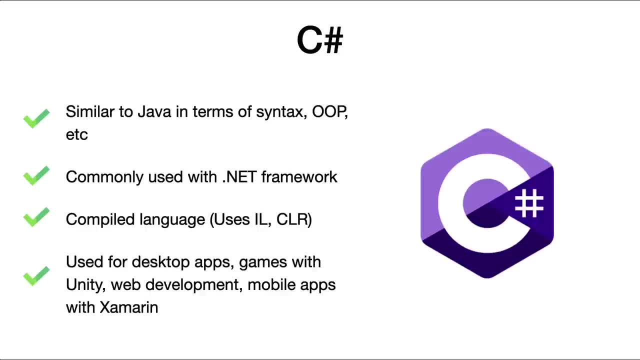 is used to build C Sharp apps, but C Sharp is also one of the languages that it was built with, including VBNET, So next we're going to look at Go or Golang, which is an extremely powerful open source language supported by Google. 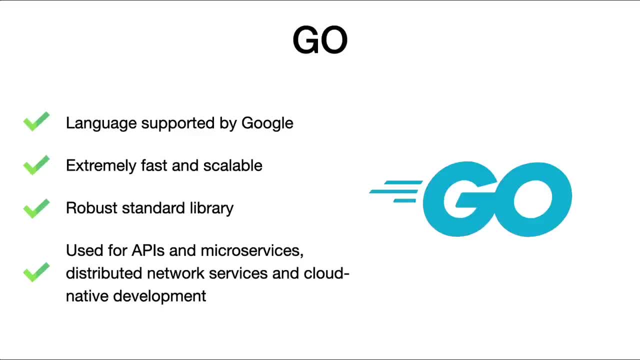 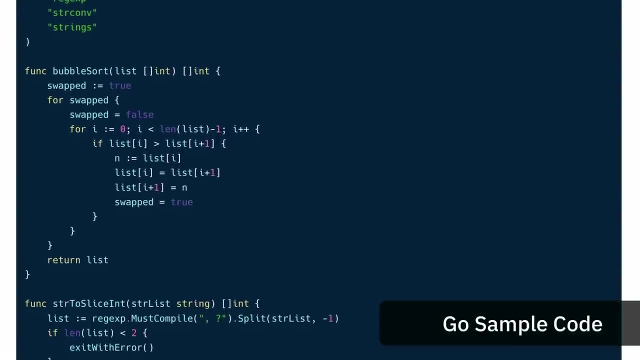 It's a compiled, statically typed language used for a lot of different things, and it's really known for being very fast and scalable, And it has a very robust standard library as well. Many parts of Go are inspired by other languages. For example, it borrows static typing. 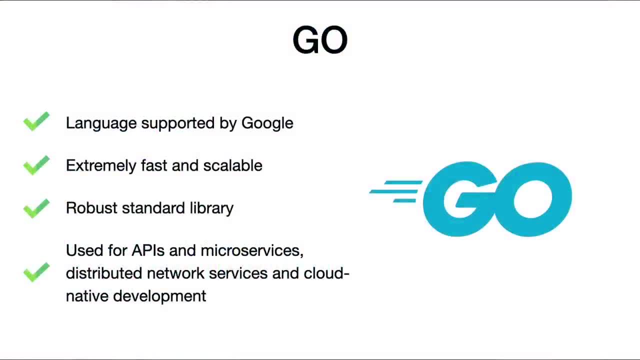 and runtime efficiency from C and its readability and usability from Python and JavaScript. So one thing I see over and over when it comes to Go programming is, like I said, it has a very robust standard library And when talking about web development, 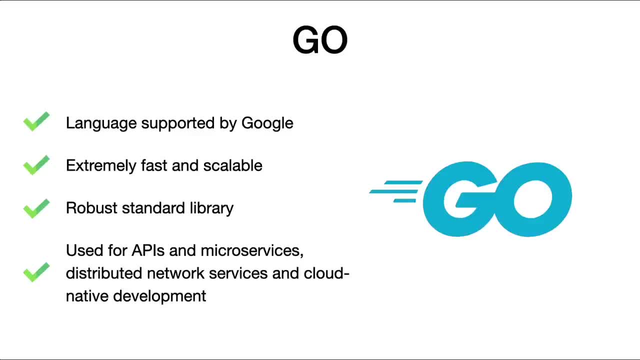 usually you use a backend framework with these types of languages if you want to build some kind of REST API or something, But with Go you actually don't need a framework for something like that. in many cases There are frameworks available, but, like I said, 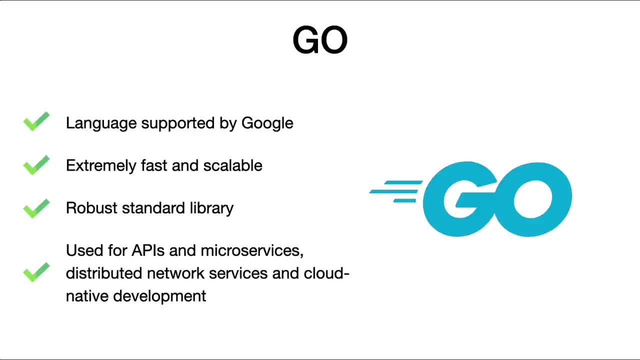 it just has a great standard library that comes with it. As far as examples of what it's used for, you have backend APIs and microservices, distributed network services and cloud-native development. Some companies that use Go are obviously Google, Uber, Dropbox. 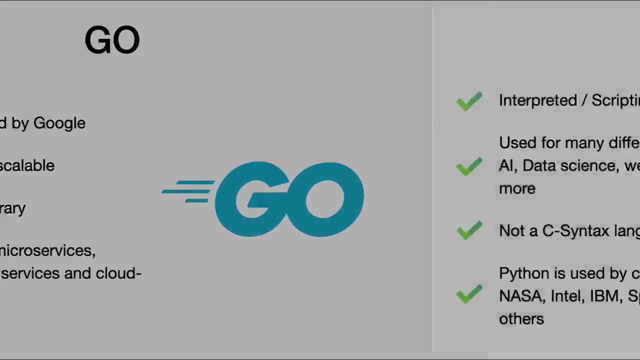 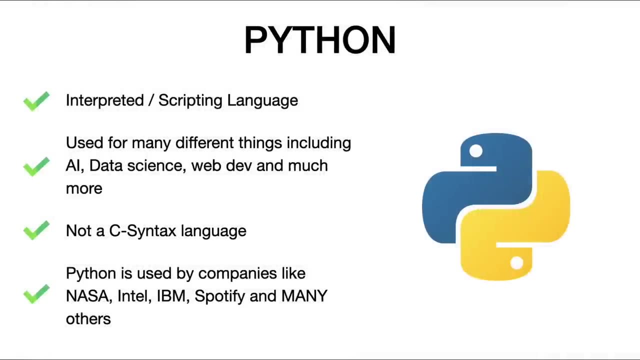 and many more. Alright, so next we're going to get into Python, which is extremely popular right now and is very diverse in its uses. So Python is a dynamic language, or dynamically typed interpreted language, also called a scripting language, And although it does, 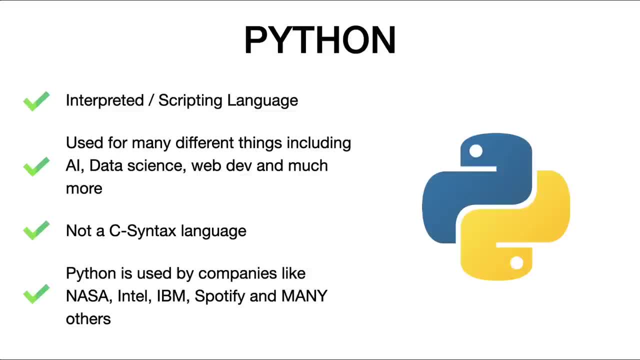 first get compiled into something called bytecode that then is executed by the interpreter, So Python is the preferred language of many developers in many different areas. It's amazing when it comes to machine learning and AI, as well as data science, automation and web development. 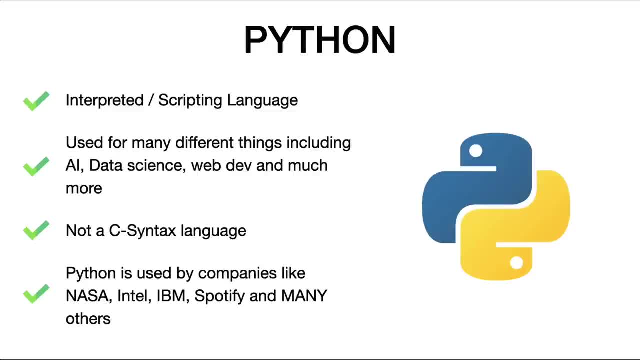 As far as web development, which is kind of my area, Python has some really great frameworks. Django and Flask, I think, are two of my top- I'd say probably my top five to seven somewhere in that range, especially Django. 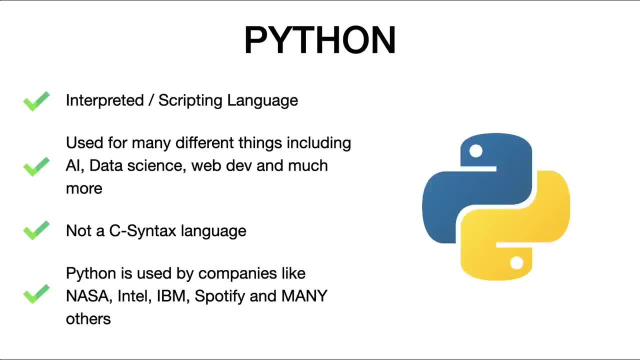 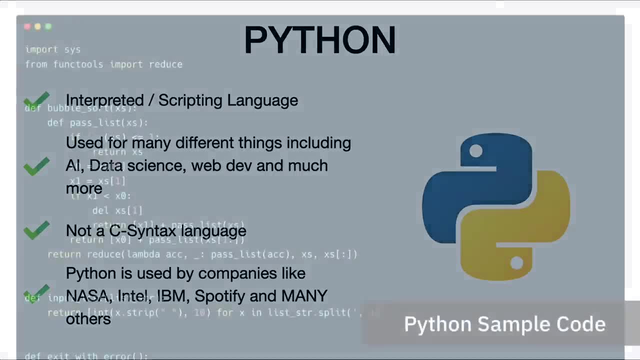 Django's probably in my top three frameworks of all time. But Python is not a C syntax language, so it looks different than something like C or Java or JavaScript. We don't use curly braces and we don't use semicolons for termination. 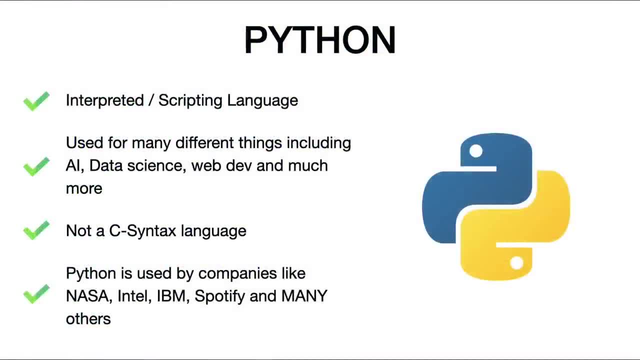 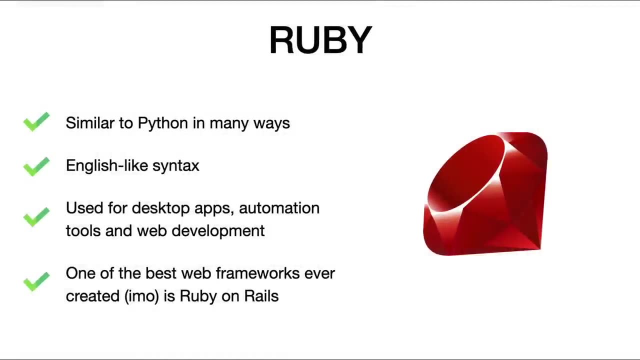 Instead we use indentation, So it looks more like plain English than many other languages. Some companies that use Python are NASA, Intel, IBM, Spotify and many other massive companies. Okay, so Ruby is a highly portable, dynamically typed language that's used for many purposes. 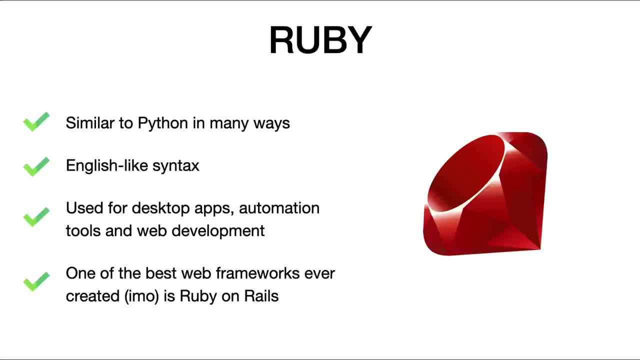 It's an interpreted languages but like Python, it's first compiled to bytecode and then interpreted by a virtual machine. I've used both Python and Ruby in my career and there seems to be a lot of similarities. They're both relatively easy to learn. 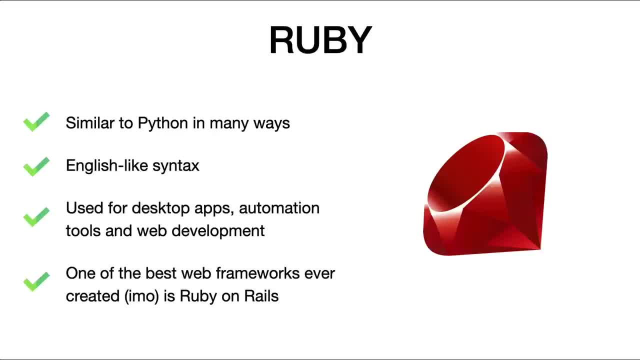 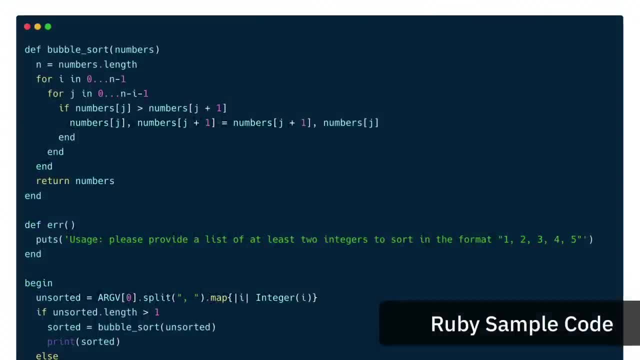 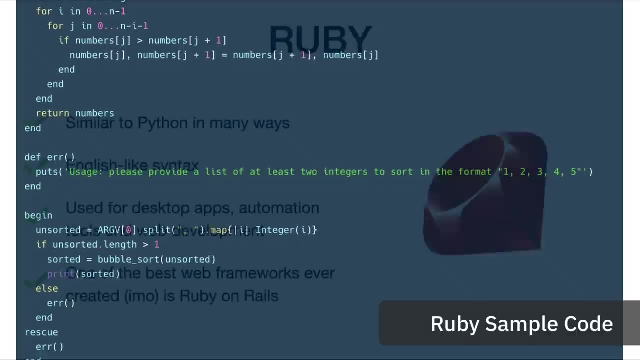 They're high-level interpreters. they're high-level interpreted languages. Python is faster than Ruby in general, but there's a lot of similarities. Ruby also doesn't use curly braces. We have the indentation syntax And the creator of Ruby, Yukihiro Matsumoto or Mats. 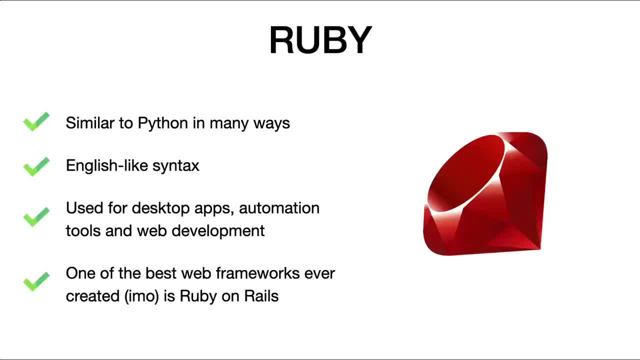 he actually said that one of his goals when creating Ruby was to make it a pretty language, a good-looking language that was easy to read and write, So it almost looks like English. So Ruby is used for building desktop applications, automation tools and web development. 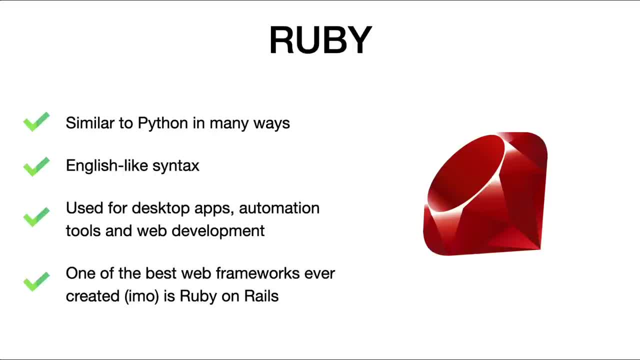 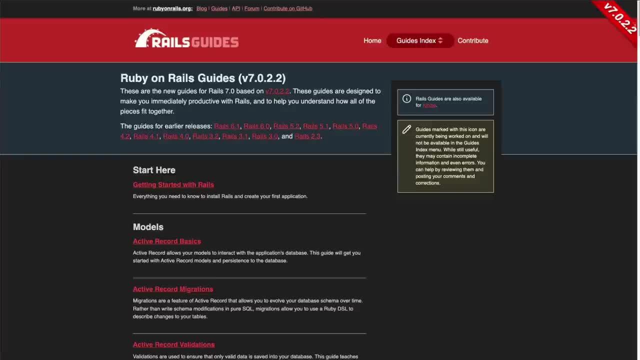 Usually, when we talk about Ruby and web development, we're talking about Ruby on Rails, which is a popular framework that I personally love and worked with for a little over a year, And it's a very opinionated framework and offers a ton of tools. 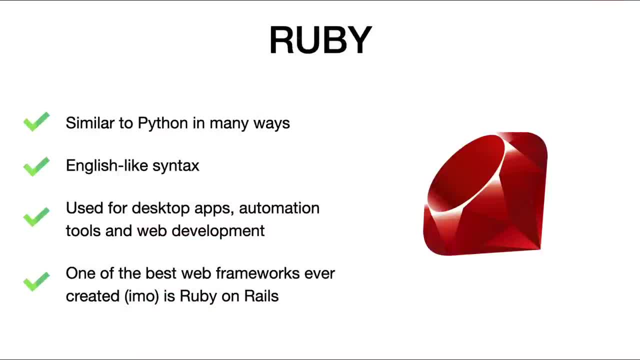 which makes it great for rapid development. So you can basically scaffold up a CRUD application that uses a database in literally a minute or two. It has lost some popularity over the last few years, but it's still a great framework Some companies that use Ruby in one way or another. 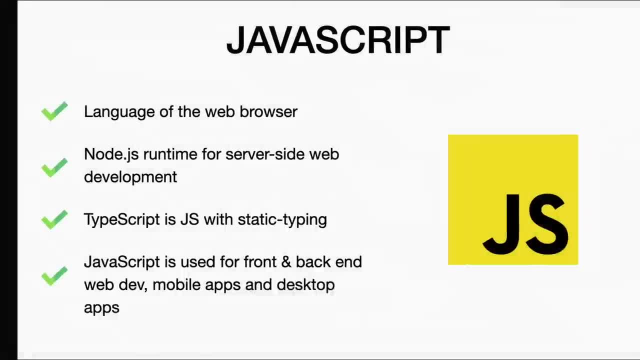 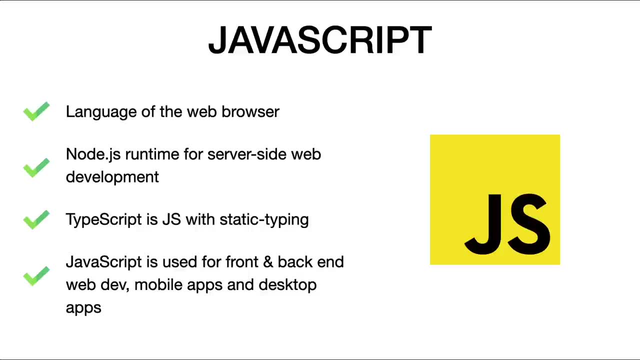 are Twitter Dribble and Groupon. All right, so now we're at the language that is very popular among my viewers and very popular in general, because JavaScript is the language of the browser. So if you're a web developer, 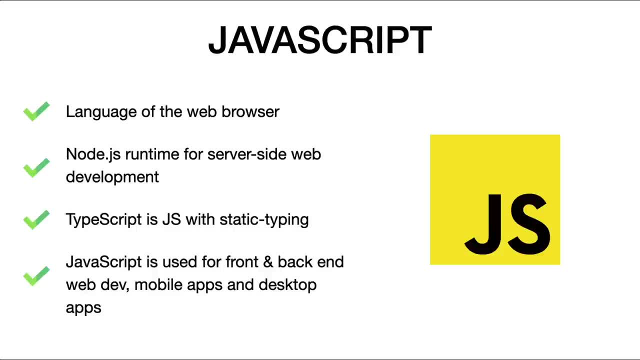 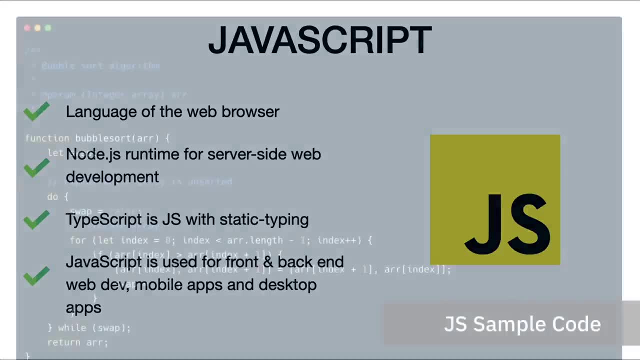 you're going to know at least some JavaScript, And it used to be. I'd say maybe like 10 years ago when JavaScript was first created, it was used to build little interactive widgets on the page, give it some dynamic properties. But over the years, 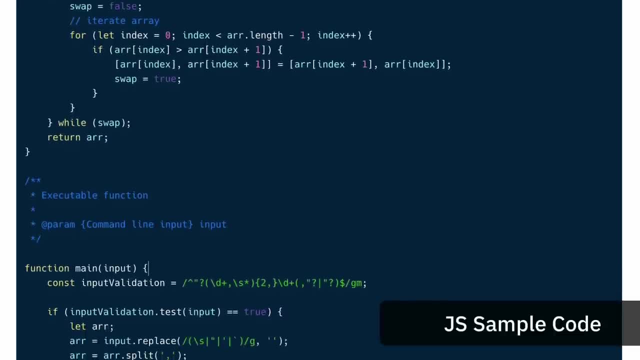 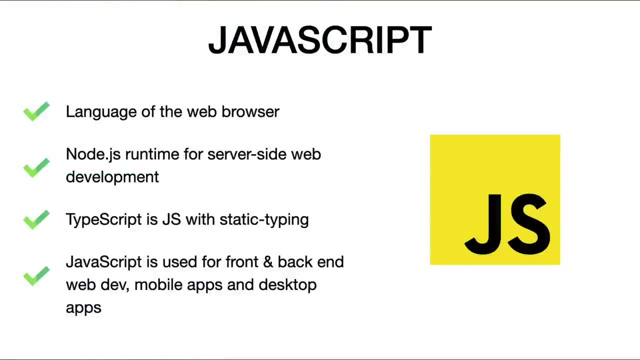 with the introduction of front-end frameworks like React, it's used for a hell of a lot more, and we can build very powerful single-page applications that run strictly on the client. And then, in addition to that, we have Nodejs, which allows us to run JavaScript on the server. 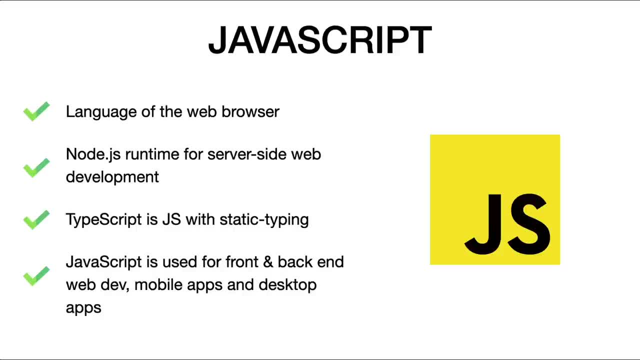 and use it just like we would any of these other back-end languages, And many full-stack developers, including myself, prefer Nodejs over other back-end solutions because they like to have the same language on the back-end as they do on the front-end. 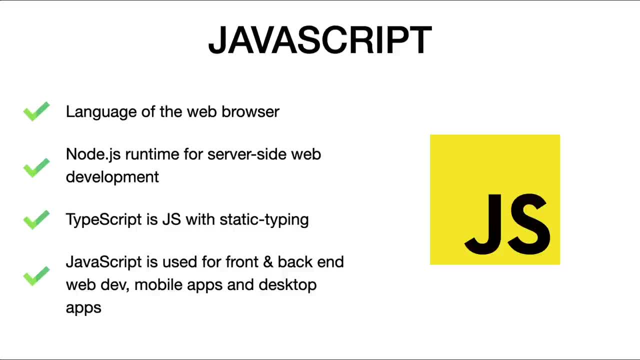 Nodejs is also extremely fast and well, at least for a lot of different tasks. it's very fast and it has a great ecosystem with NPM, which is the Node Package Manager. So JavaScript is an interpreted scripting language that by default, 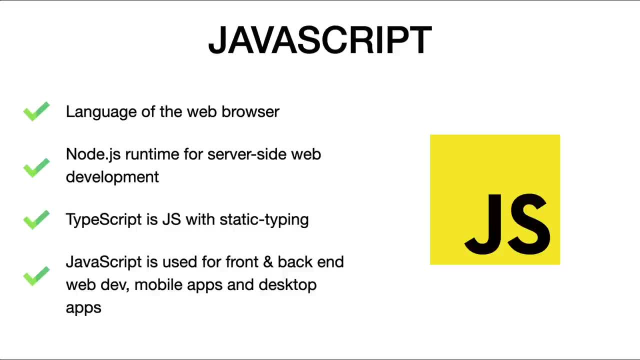 is dynamic, but if you want, you can use TypeScript, which is a superset of JavaScript that adds static typing. So front-end JavaScript is used by just about every company that does anything in the browser, and Nodejs, or back-end JavaScript, is used by companies like NASA. 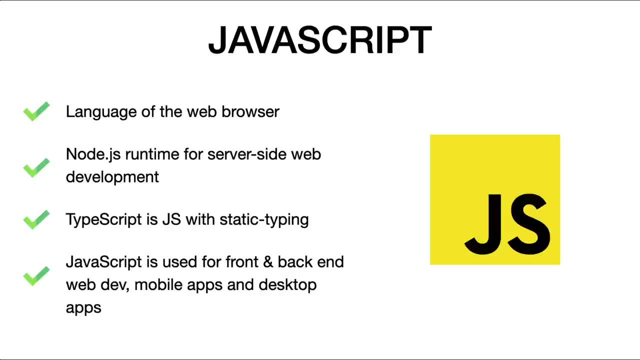 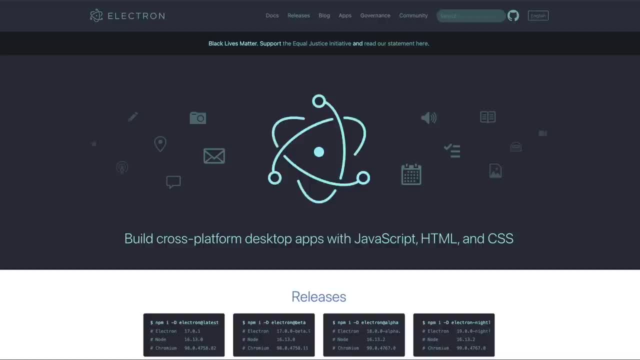 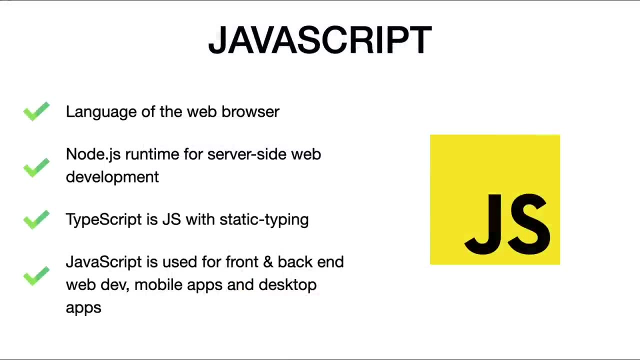 PayPal, Medium and Netflix. We also have technologies like React Native that lets us use JavaScript to build mobile applications, And then we have Electron, as well as some other frameworks that allow us to use JavaScript to build desktop applications. In fact, VS Code is built with JavaScript. 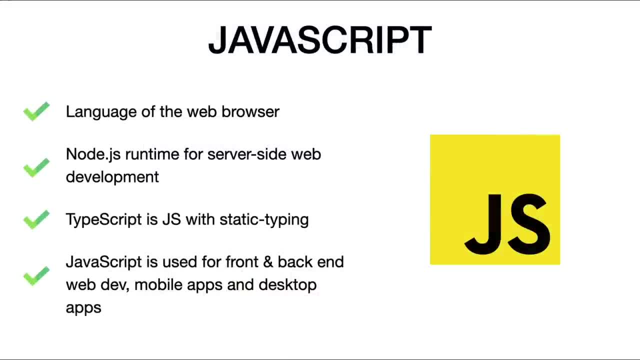 as well as some other popular desktop apps such as Postman and Slack, So JavaScript is absolutely everywhere, which is another reason that I love it All right, so next we're going to look at PHP, which is actually the first language that I really learned. 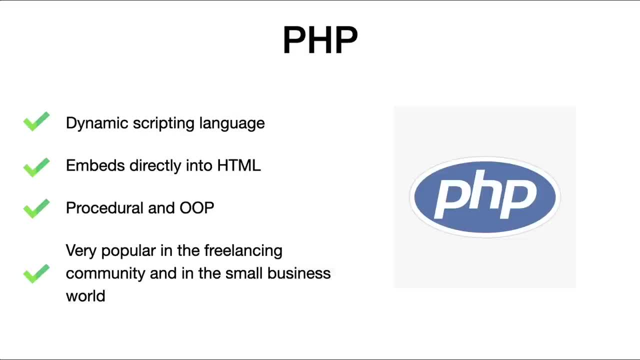 Java was the first language that I ever used, but I stopped when I decided to go into web dev because PHP was so popular at the time. So PHP is a dynamic scripting language that is used to build static and dynamic websites and web apps. 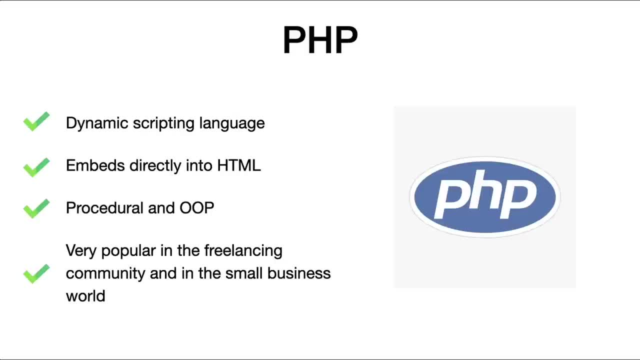 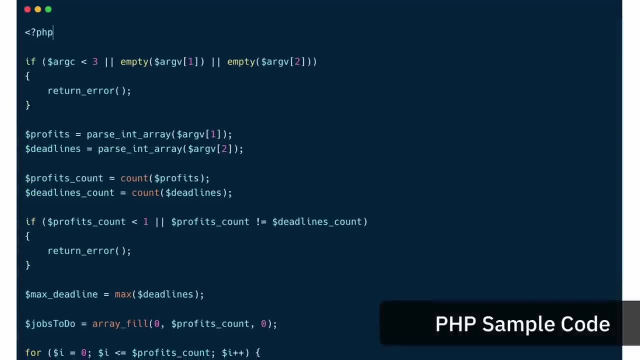 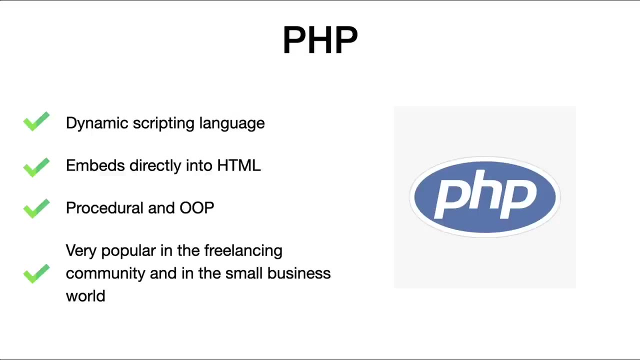 And what's really cool about PHP and makes it very practical for web developers is that you can embed PHP directly into directly with HTML, And that makes it easy to add functionality to websites without having to call external files. So PHP can be used as a procedure. 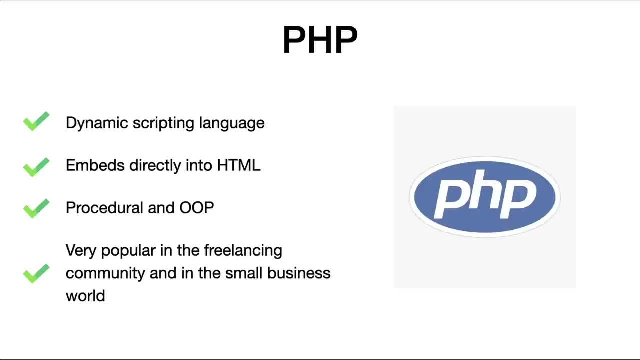 or as an object-oriented language. The syntax can sometimes be pretty messy. I think that it gets a lot of flack for that, So I do prefer to use it in an object-oriented way. I think that makes it much cleaner. There are some great frameworks. 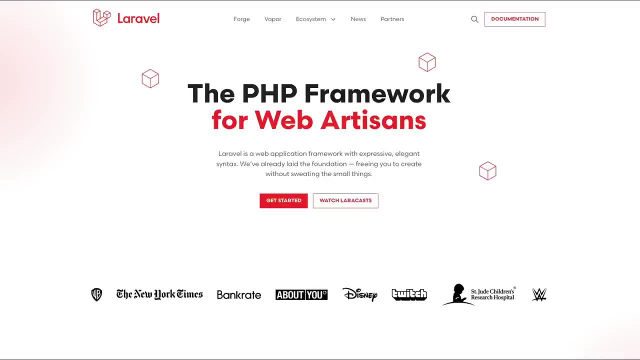 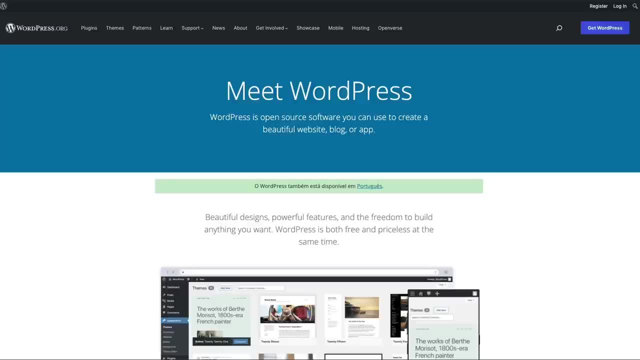 web frameworks for PHP, such as Laravel, And there's all types of open-source tools like WordPress, which is a blogging platform or CMS. So PHP is great for making things fast, which makes it easy to use. It makes it really popular in the freelancing community. 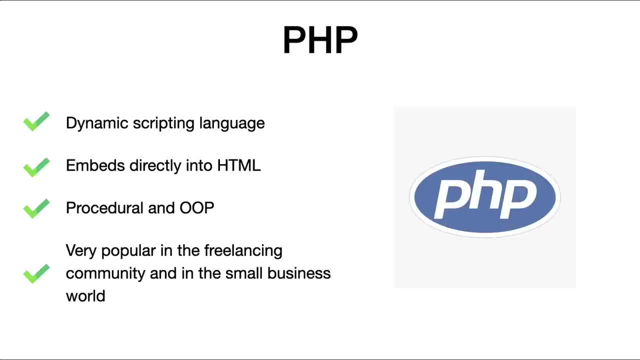 as well as small businesses. There's quite a bit of hate online towards PHP, but it's getting better. Part of the reason of that is I think PHP is getting better now with version 8. And it's usually from people that never really worked with it. 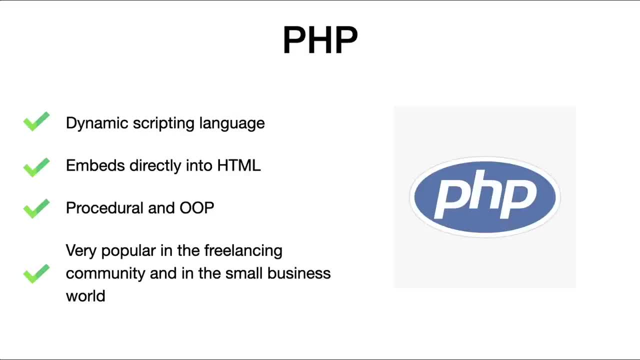 or haven't worked with it for a while or have never worked as a freelancer or outside of a big company on a team, Because, again, PHP is great for just building things fast and getting products out there All right. So Swift is a general-purpose. 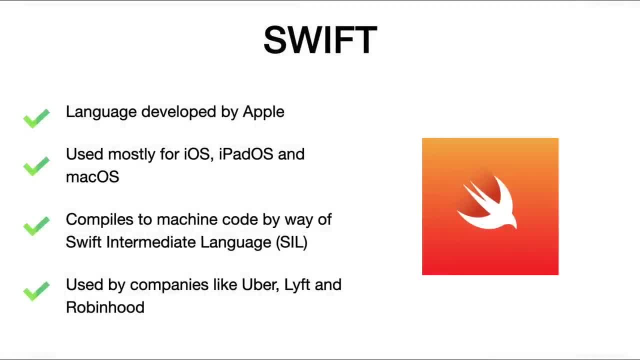 compiled language developed by Apple and is mostly used to develop applications for iOS, iPadOS, MacOS and any other device that Apple creates. It's relatively easy to learn and it's extremely fast. iPhone applications used to be created mostly with a language called Objective-C. 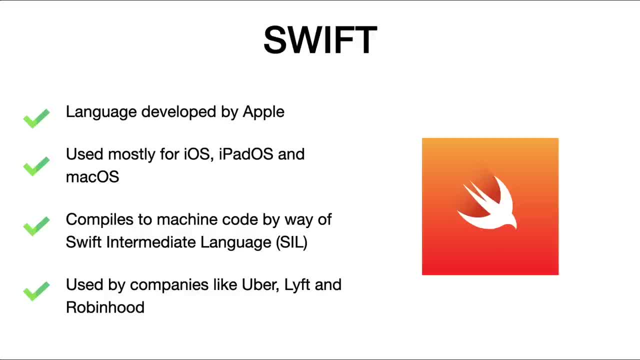 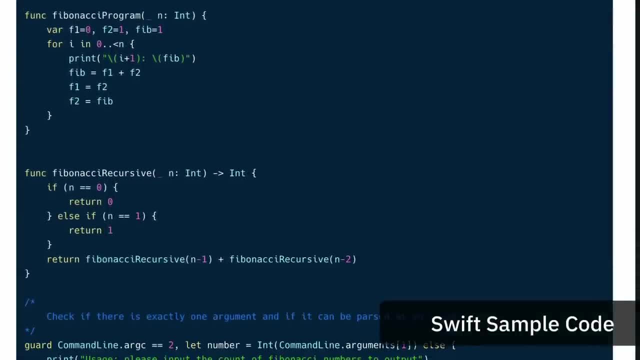 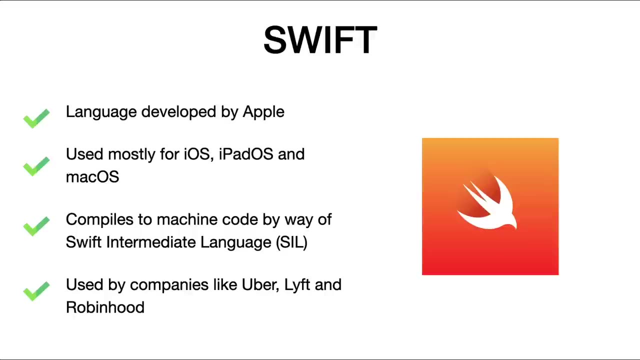 but most are built with Swift these days And I believe Apple has stated that Swift is about 2.5 times faster than Objective-C. So if you're looking or thinking of going into native iOS apps or MacOS, Swift is one of your main choices. 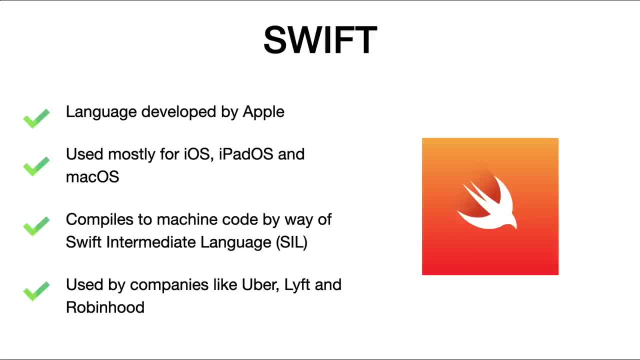 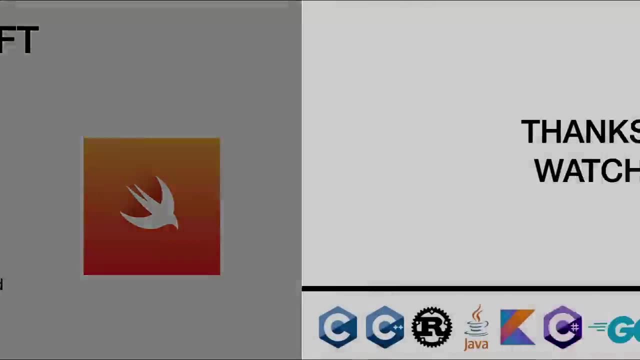 Like I said, Swift is very fast and it's first compiled into something called Swift Intermediate Language and then into machine code, from what I understand, And companies like Uber, Robinhood and Lyft all use Swift in their tech stacks. All right. 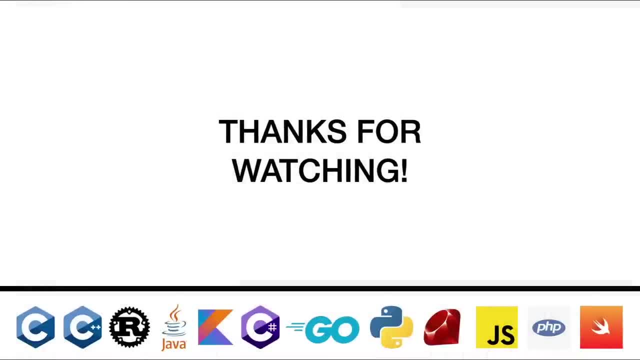 So obviously there's other programming languages out there, but I think that these are some of the most popular ones, at least at this time, And, as you can see, they're all very different. So what I would suggest is: just look at what you want to do in tech. 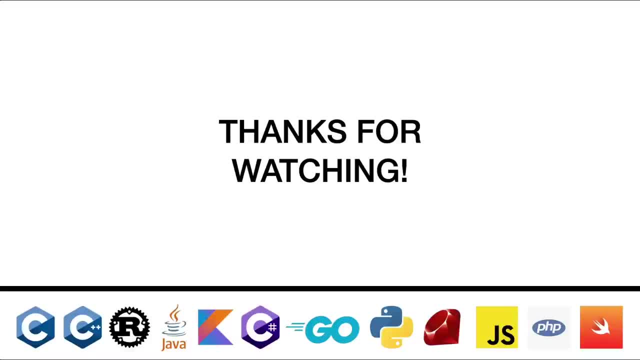 and find a language that best suits you. You may have to try a few languages, but that's fine, Even if you learn, let's say, the basics in Ruby. if you switch to Python, there'll be a lot that you can grasp very quickly. 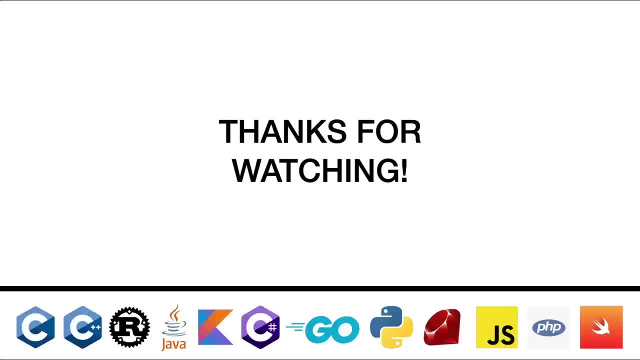 because of what you learned in Ruby, And a lot of it comes down to syntax, but I also wanted you to just get familiar with what high level languages are and low level and static and dynamic typing and all that good stuff. So I hope you learned something from this video. and thanks for watching and I'll see you next time.